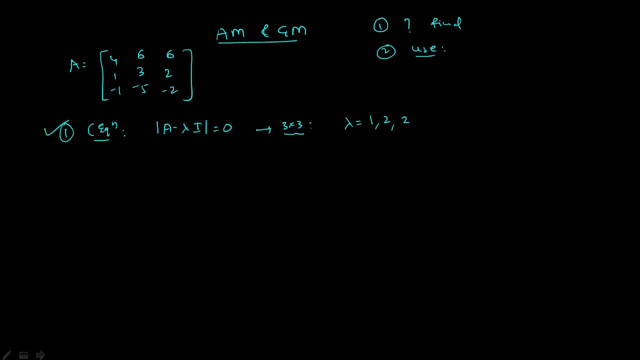 Now my question is: if you don't know how to do this part first step, please do watch my previous video, Then you can get this first step. Now let's move forward to the next part. So this is the main topic of am and gm. So second point is about that. 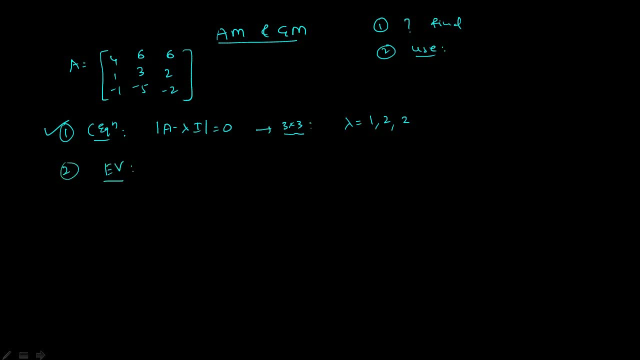 Now we have to find the eigenvector. Eigenvector is important to find am and gm. Okay, how to find eigenvector, For lambda is equal to 1, what is the respective matrix Matrix of a minus lambda i, where lambda value is 1 and, into capital, X is equal to 0. 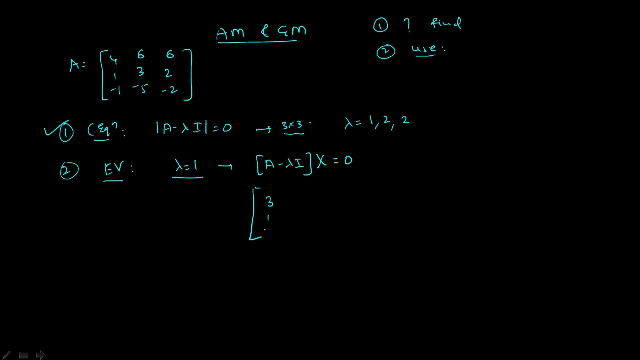 So after doing that, the matrix you will get here as 3, 1 minus 1,, 6, 2 minus 5, then 6, 2 minus 3 and X can be represented as 3 variables: X1, X2 and X3. 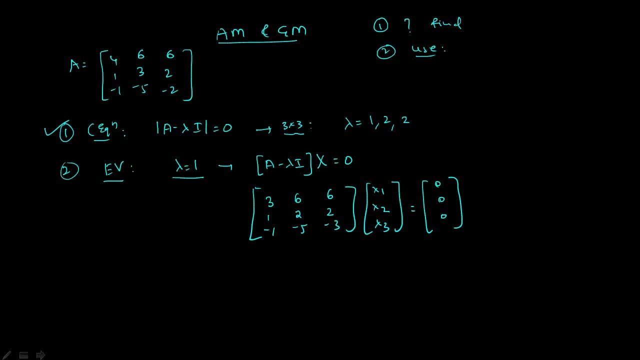 0 can be represented in the matrix form as this: Okay, so now we have to do the manipulation to arrive at the answer. So first I will do the row 1 as row 1 by 2.. So because it is divisible, row 1 by 3, because it is divisible by 3.. 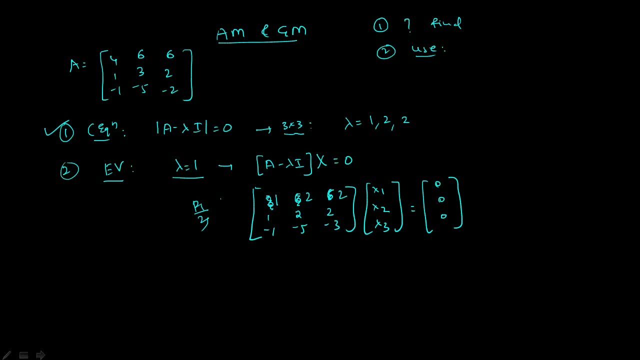 So this will be 1, this would be 2, this would be 2, and now, because row 1 and row 2 are equal, I can change the row 2 as row 1 minus row 2, and now I will get. the row 1 is unaffected. 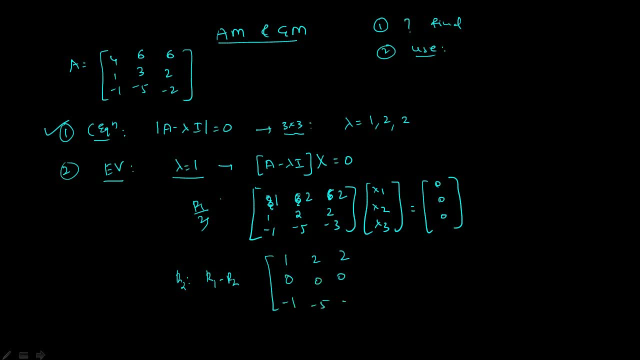 Row 2 has changed to 0 and the last row is as it is and the rest part, But now I can make this term as 0 as well. How I will? let me take it here. What I will do is I will change the row 3 as row 3 plus row 1.. 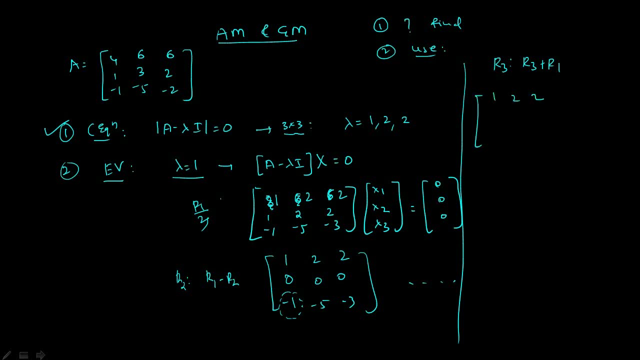 If I do that, row 1 is still unaffected, 1 to 2, row 2 has become 0 and now row 3 will change, So it would be 0, then minus 3, then minus 1, and the x can be represented as this: and the 0 matrix. 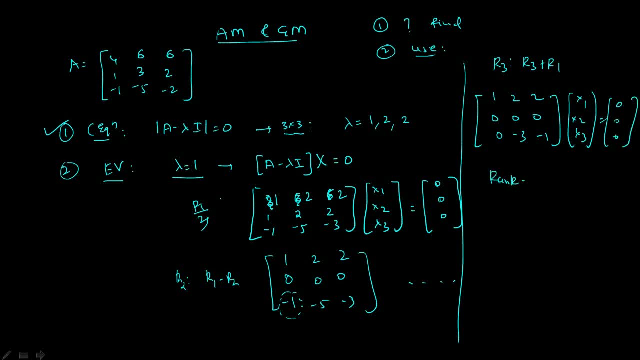 Okay, now we can say that our rank is equal to 2, because rank is equal to number of non-zero rows. So how many non-zero rows? we have 2, which is r1 and r3.. So rank is 2.. 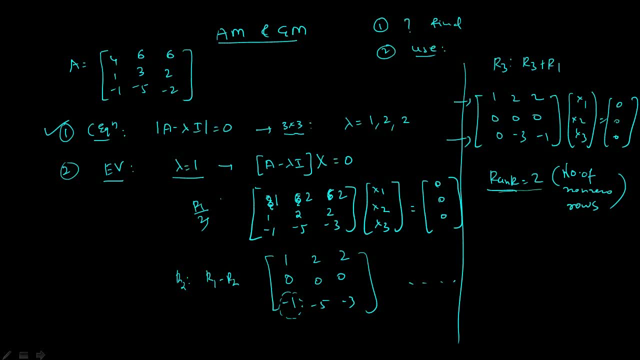 Now why this rank is important in am-gm concept. Now you will understand. because gm is equal to number of variables minus rank. So number of variable is this. So 3 variable we have, Rank is 2.. So gm is 1.. 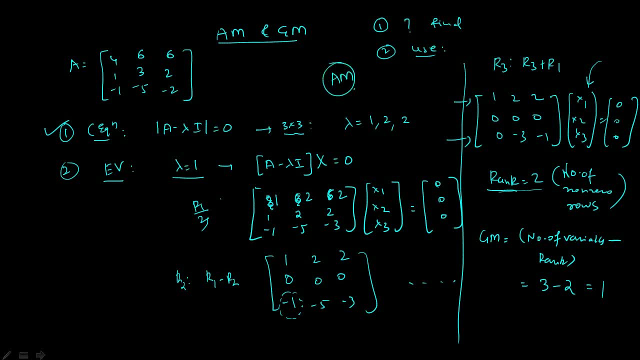 Now, when we talk about am, am is found by here. So for lambda is equal to 1, am is 1.. And for lambda is equal to 2, am is 2.. Because lambda means meaning of that. lambda means number of times, number of times lambda repeats. 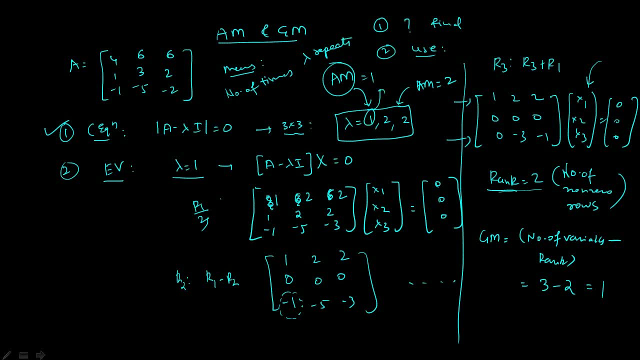 So 1 is repeated only 1 time, but 2 is repeated 2 times, So am is 2.. Okay, So here the case is simple, For lambda is equal to 1, am is 1, because lambda equal to 1 is only 1 time. 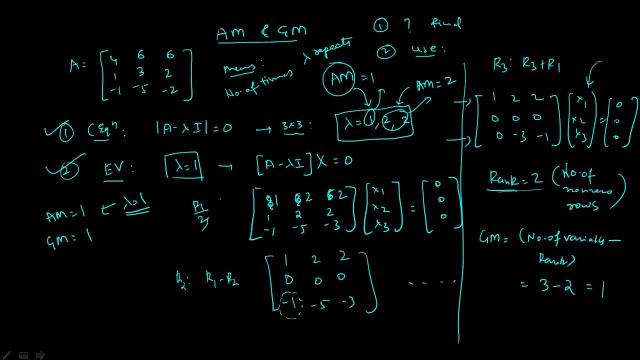 And gm is equal to 1, because we saw the calculation. So this is how we can learn about am and gm, how we can find that And if you have learned it correctly, then tell me, for lambda is equal to 2.. 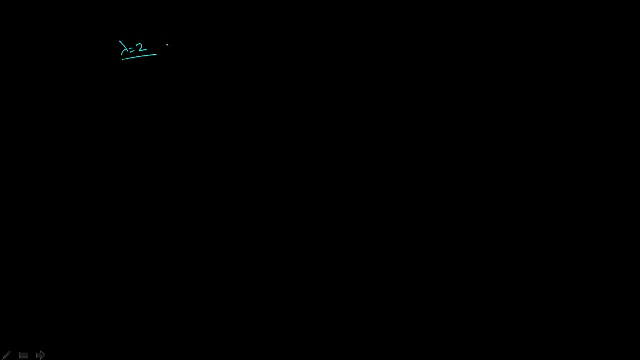 So if we move forward, for lambda is equal to 2, the respective eigenvector you have to find and you have to do the further calculation, Which I won't do. I expect you can do it And if you do that you will find that am is 2.. 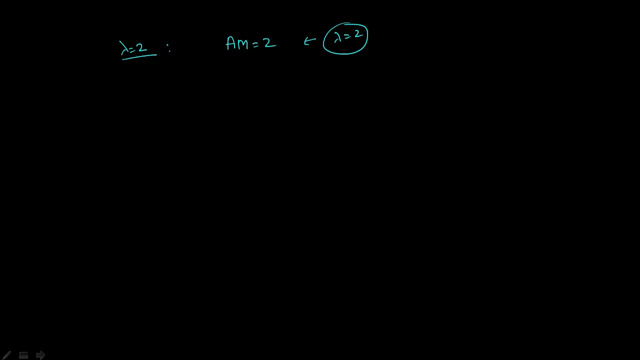 Because lambda is equal to 2 is repeated 2 times. When we found the lambda value from the characteristic equation, It was 1 to 2.. So 2 is repeated 2 times, So am is 2.. Now let's talk about gm. 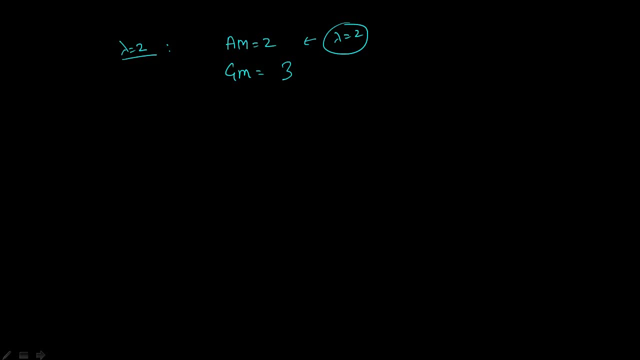 gm. after you do the same procedure, that variable is 3, but what was the rank? And you will find that the rank is 2.. Okay, So if rank is 2, then you will get the geometric multiplicity as 1.. 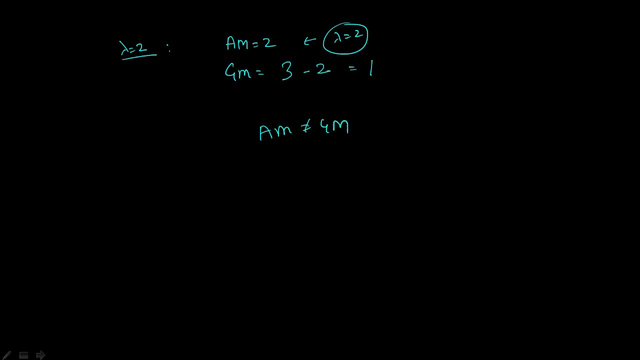 And you can see that am is not equal to gm. So this is important, Because in lambda is equal to 1, am was equal to gm, Correct, And both of the values were 1.. So what is the case here and how we can proceed in the usage.